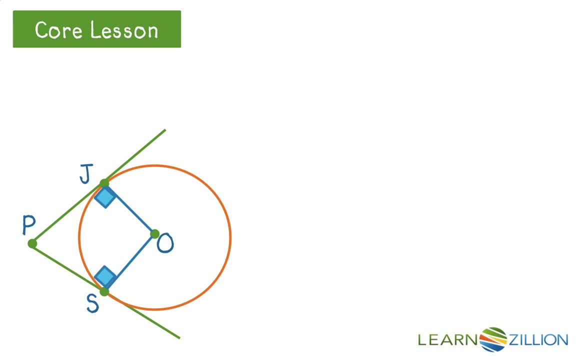 First, we notice that we have right angles where the tangents and radii intersect, based on a previous theorem. We also notice that OJPS is a quadrilateral and more than that a kite, because we know that there are segments that are congruent from our tangent theorems. 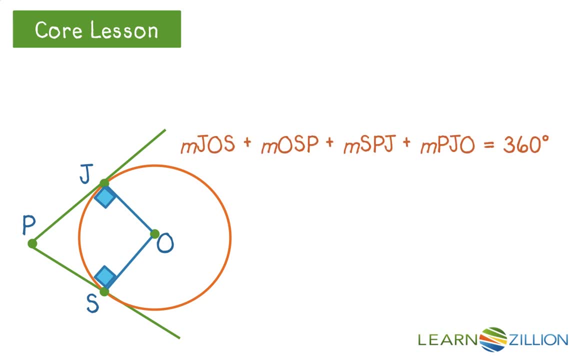 We also know the quadrilaterals have angle measurements that sum to 360 degrees. Using that, we have two right angles. we can replace angle measure OSP and angle measure PJO with 90 degrees. Then, combining like terms, we have 180 degrees. 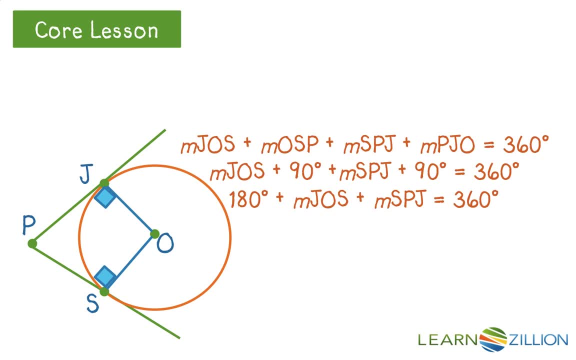 plus our two remaining angle measures gives us 360 degrees. Subtracting 180 degrees from both sides, we have that angle measure JOS, the central angle, plus angle measure SPJ, the circumscribed angle sum to 180 degrees. 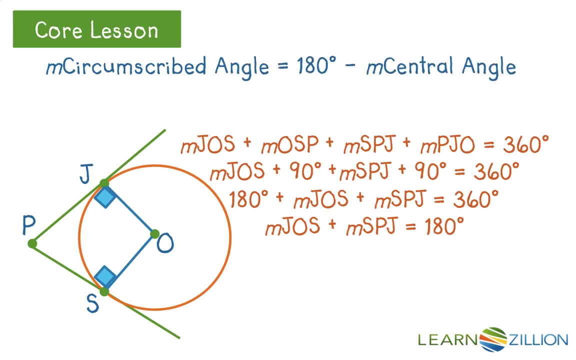 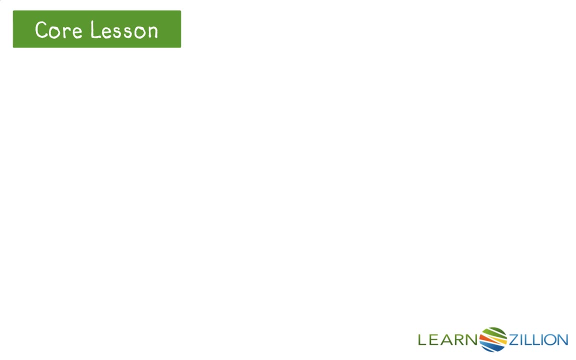 This tells us that the measure of the circumscribed angle is 180 degrees minus the measure of the central angle. It also tells us that the measure of a central angle is 180 degrees minus the measure of a circumscribed angle. Let's look at an example. 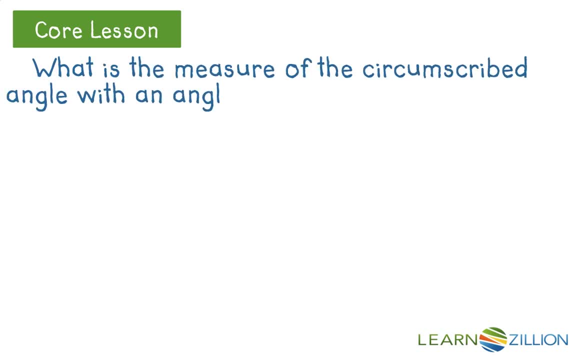 What is the measure of the circumscribed angle whose intercepted arc has a measure of 60 degrees? Well, looking at a diagram, we have a circumscribed angle and have labeled the arc measure: 60 degrees. We know that we can use our derived formula. 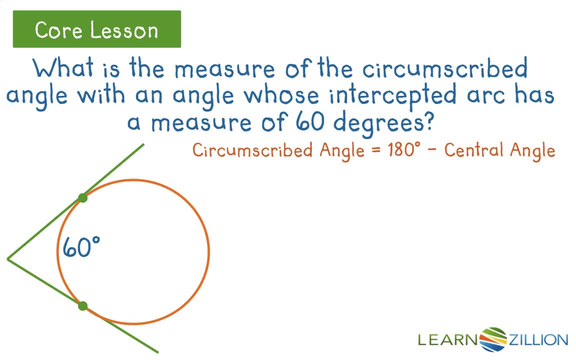 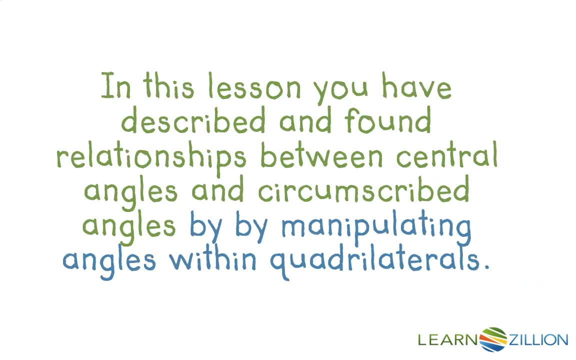 to solve the problem. We also need to use information from our last lesson to know that the central angle measure and arc measure are congruent. So with the substitution we can see that the measure of the circumscribed angle is 120 degrees. 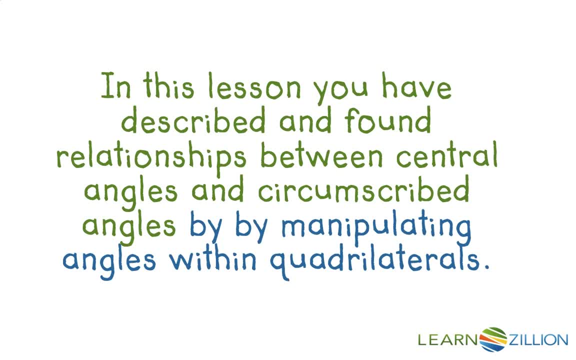 In this lesson you have described and found relationships between central angles and circumscribed angles by manipulating angles within quadrilaterals.